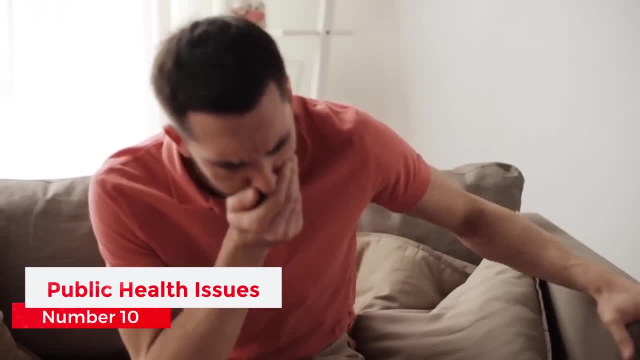 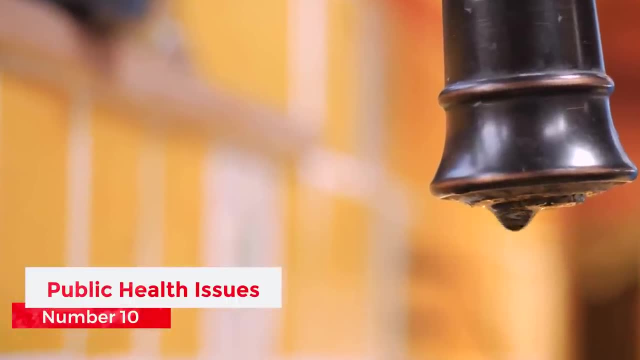 sanitation and hygiene-related diseases, which could be reduced with safe water and sanitation access. Every two minutes, a child dies from a water-related illness. Access to safe water and sanitation contributes to the health of the population. 10. Public Health Issues. 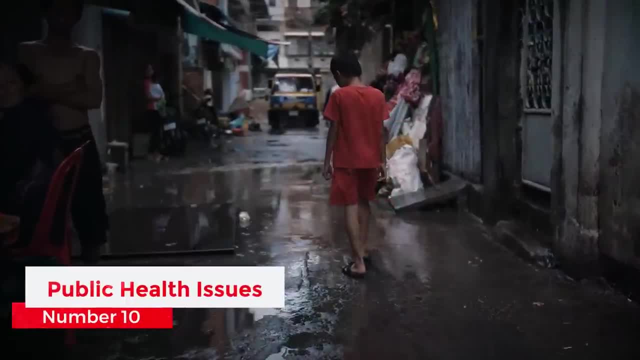 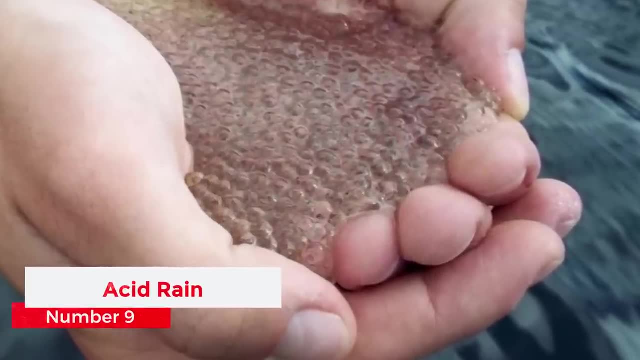 COVID-19 has contributed to the health of the population and has helped prevent the spread of infectious diseases. 9. Acid Rain: Acid rain is not pure acid falling from the sky, but rather it is rainfall or atmospheric moisture that has been mixed with elements and gases that have caused the moisture to 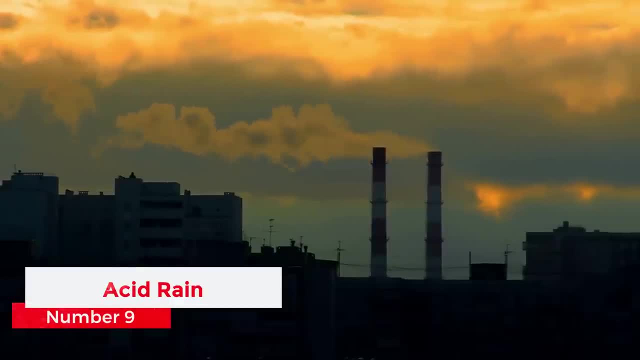 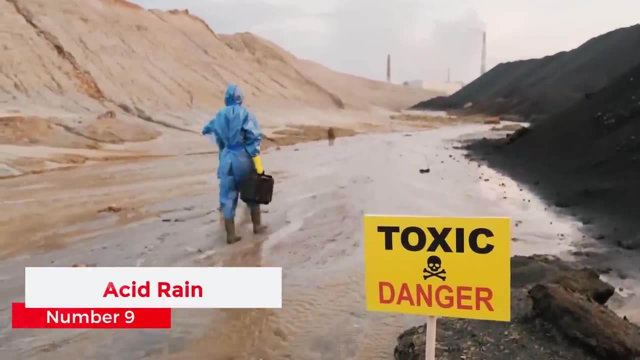 become more acidic than normal. Acidic precipitation can be caused by natural volcanoes or man-made activities such as cars and electricity generation. Air pollution like sulfur dioxide and nitrogen oxides can cause acidification. It can cause respiratory diseases or worsen these diseases. Acid rain can be extremely. 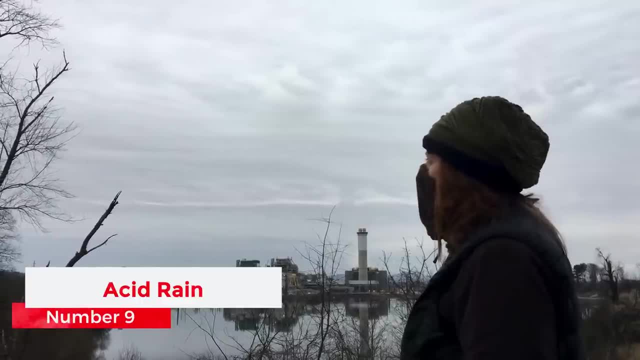 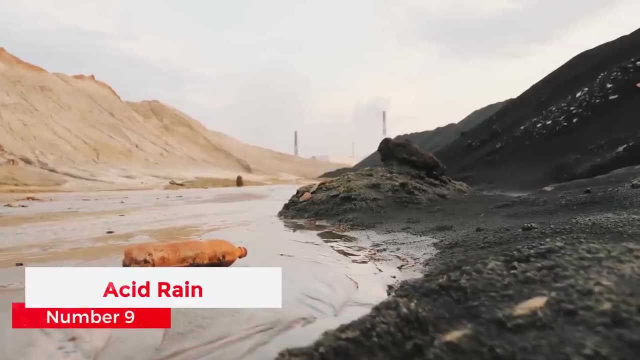 harmful to forests too. Acid rain that seeps into the ground can dissolve nutrients such as magnesium and calcium that trees need to be healthy. Another thing: When acid rain and dry acidic particles fall to earth, the nitric and sulfuric 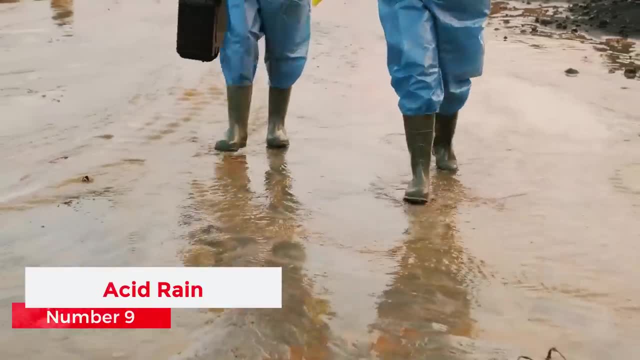 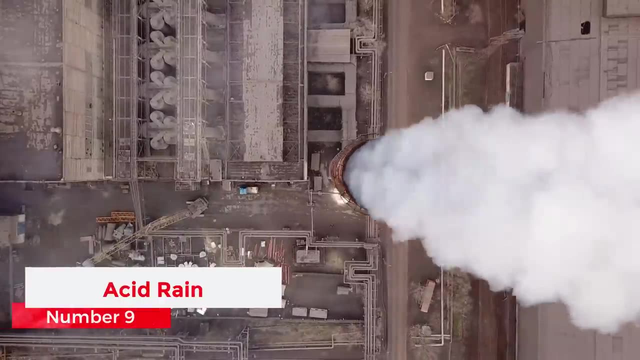 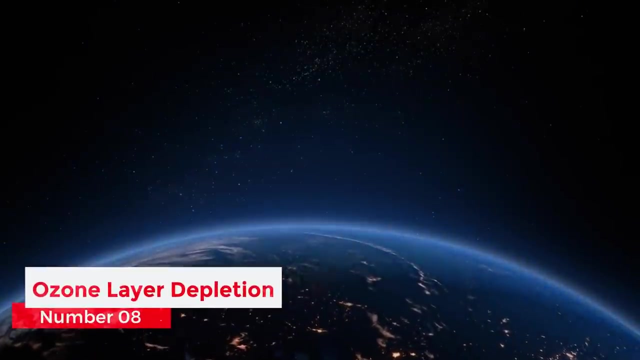 acid that makes the particles acidic can land on statues, buildings and other man-made structures and damage their surfaces. The acidic particles corrode metal and cause paint and stone to deteriorate more quickly. 8. Ozone Layer Depletion. The ozone layer is a layer of gas present in the uppermost part of the atmosphere. It 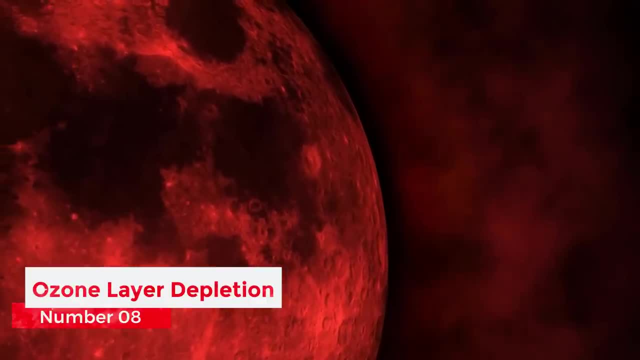 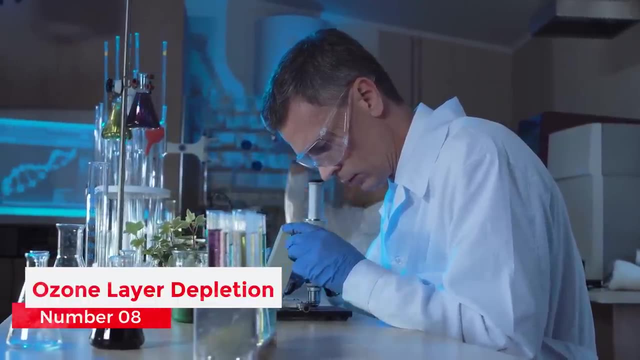 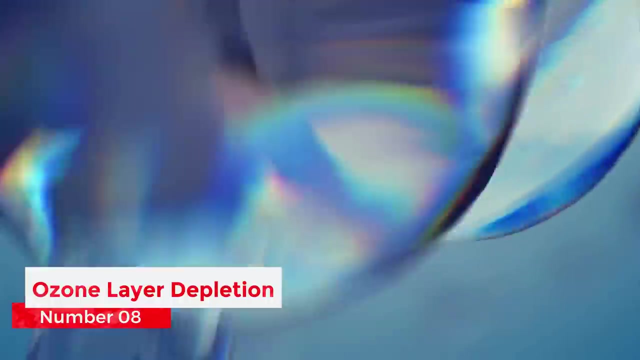 protects the planet by stopping the UV rays that are coming from the sun. Ozone layer depletion increases the amount of UBV that reaches the earth's surface. Laboratory and epidemiological studies demonstrate that UVB causes non-melanoma skin cancer and plays a significant role in malignant melanoma development. In addition, UVB has been linked to the development 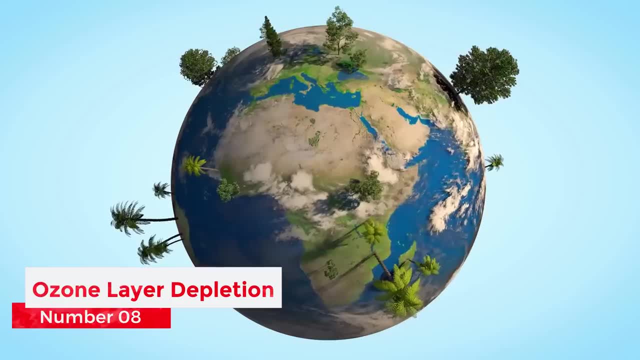 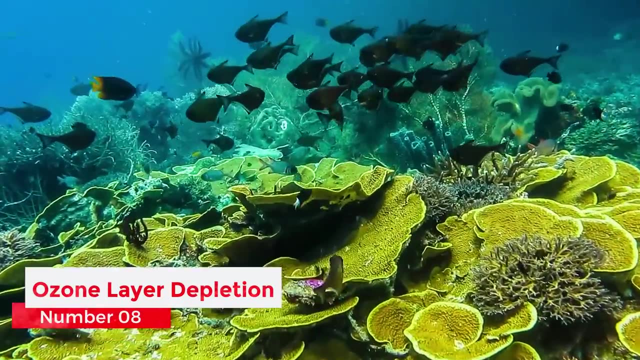 of cataracts. In addition to that, UVB radiation has been found to cause damage to the early developmental stages of fish, shrimp, crab, amphibians and other marine animals. The most severe effects are decreased reproductive capacity and impaired larval development. It has major 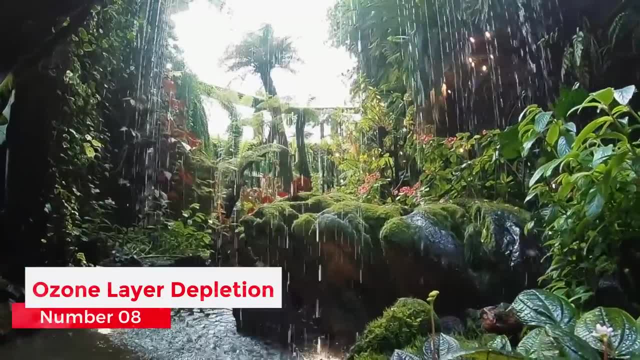 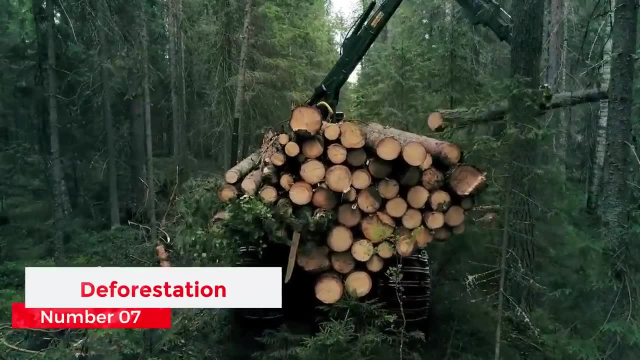 effects too, on plants, biogeochemical cycles, to materials as well. 7. Deforestation: Deforestation simply means clearing green cover and making that land available for residential, industrial or commercial use. It is a very important part of the life of a human being. 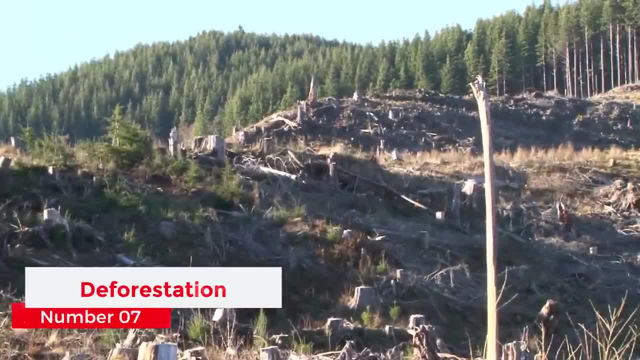 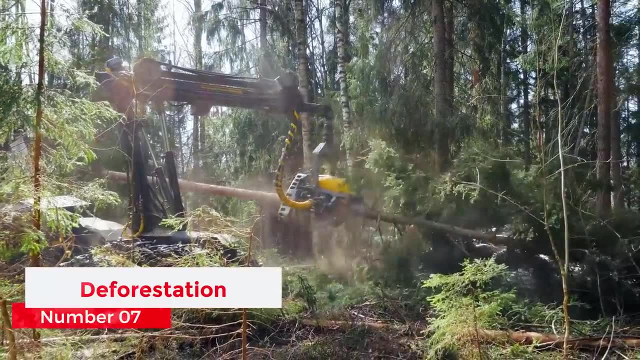 Our forests are natural sinks of carbon dioxide and produce fresh oxygen. They also help regulate temperature and rainfall. But every minute, forests the size of 20 football fields are cut down. By 2030, the planet might have only 10% of its forests If deforestation isn't. 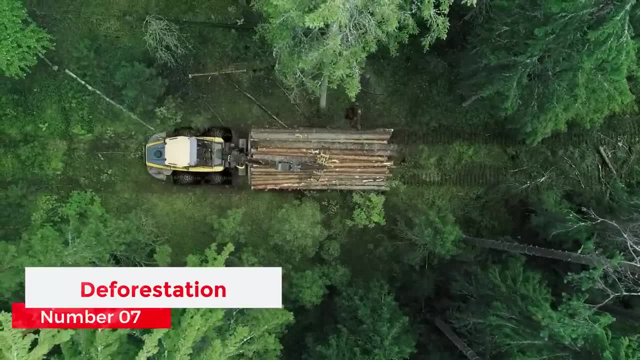 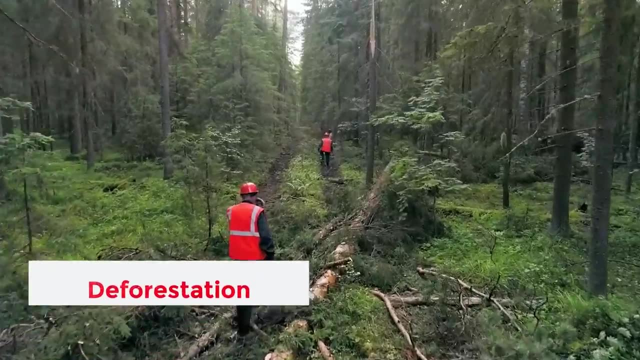 stopped, they could all be gone in less than a hundred years. Soil erosion, irregular rains, flooding, increased greenhouse gases are some of the adverse effects this has on our environment. 6. Loss of Biodiversity. Loss of biodiversity is one of the most common causes of deforestation in the world. The 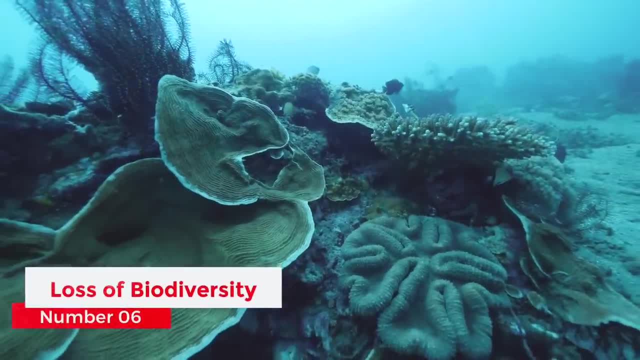 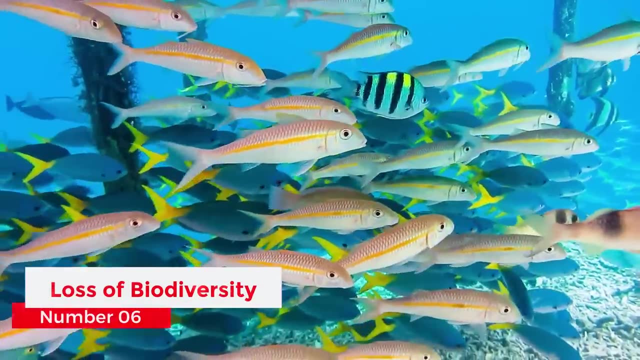 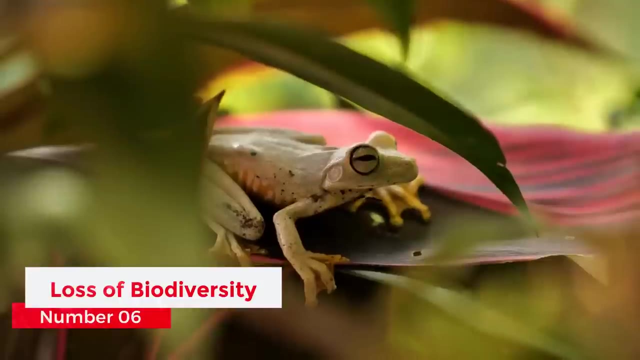 loss of biodiversity refers to the decline or disappearance of biological diversity, understood as the variety of living things that inhabit the planet. Human activity is leading to the extinction of species and habitats and loss of biodiversity. Ecosystems which took millions of years to perfect are in danger when any species population is decimating Biodiversity. 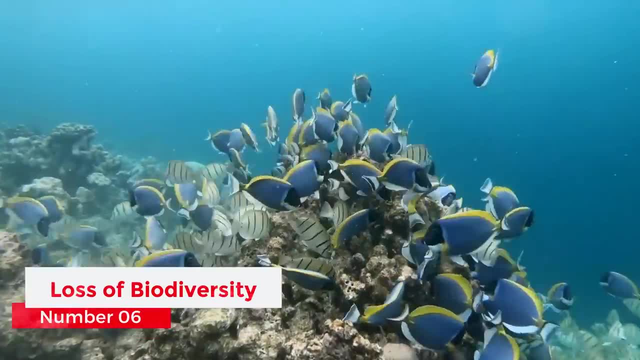 is essential because every species on the earth is helpful to keep many ecosystems healthy, thriving and balanced. It plays a vital role in the sustainable development of the environment. 7. Loss of Biodiversity- Loss of biodiversity- plays a vital role in the sustainability of life on earth. More. 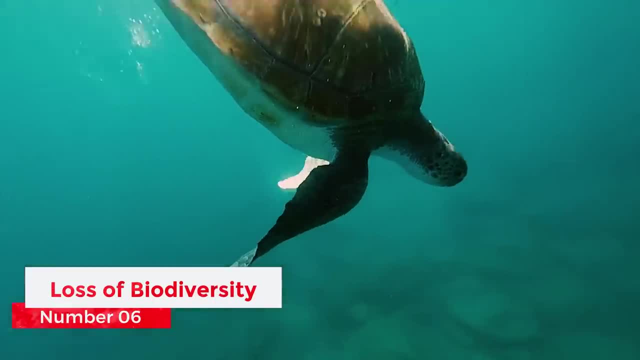 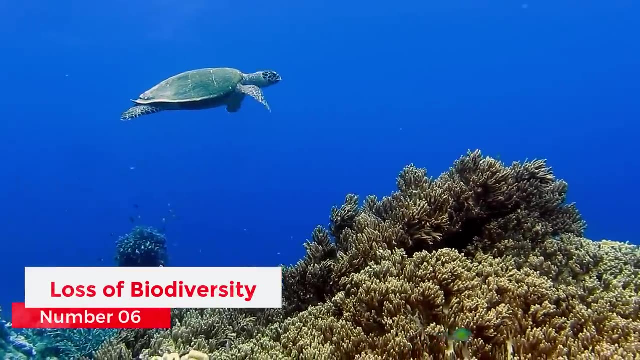 than 500 species of land animals are on the brink of extinction and are likely to be lost within 20 years. the same number were lost over the whole of the last century. Many species have experienced substantial losses and many are nearing extinction, so awareness is essential. 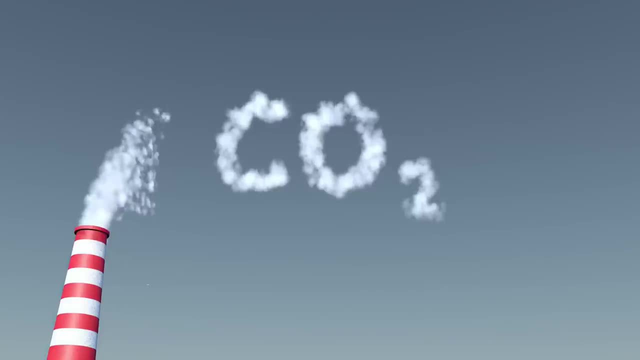 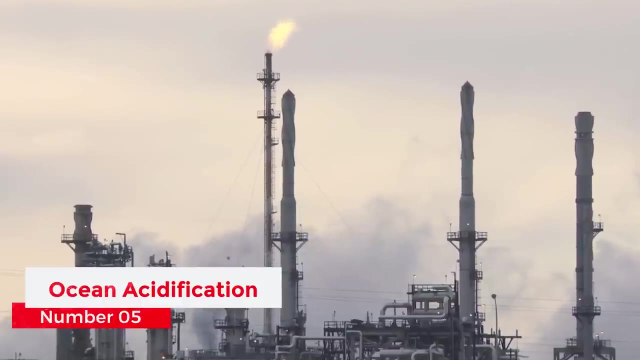 to control it. 5. Ocean Acidification: Human activities release CO2 into the atmosphere, which leads to atmospheric warming and climate change. Around a third to a half of the world's oceanic resources are polluted by CO2.. This, compared to the amount of CO2 released by human activities, is absorbed into the oceans. 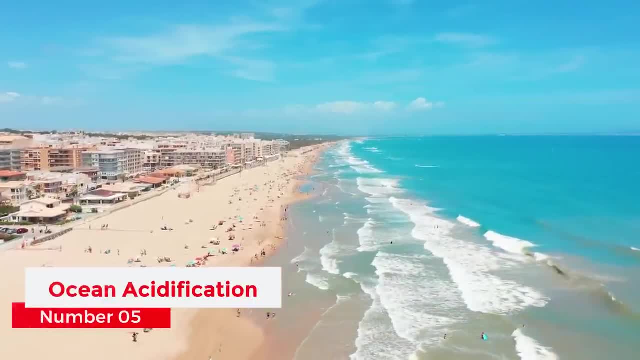 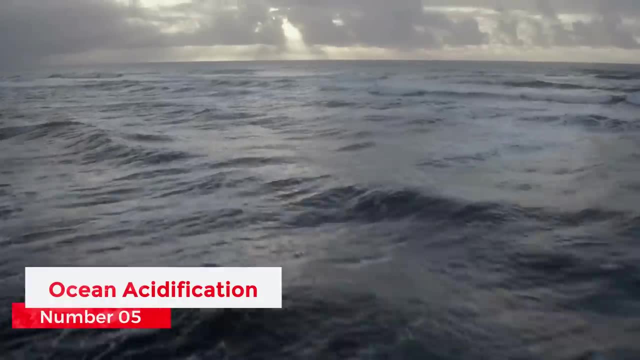 While this helps reduce the rate of atmospheric warming and climate change, it also has a direct chemical effect on seawater, which we call ocean acidification. Due to this, the pH level of the seawater increases, affecting marine life and coral reefs. so controlling 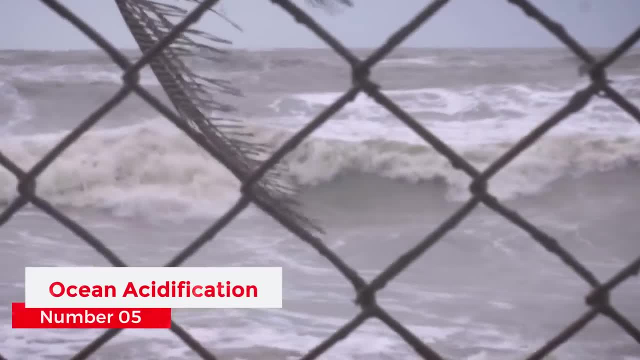 the amount of CO2 in our atmosphere will also help our oceans sustain life. 4. Waste Disposal, The over-consumption of resources and the creation of plastic waste and natural resources are the main reasons for the increase in the amount of CO2 released by human activities in. 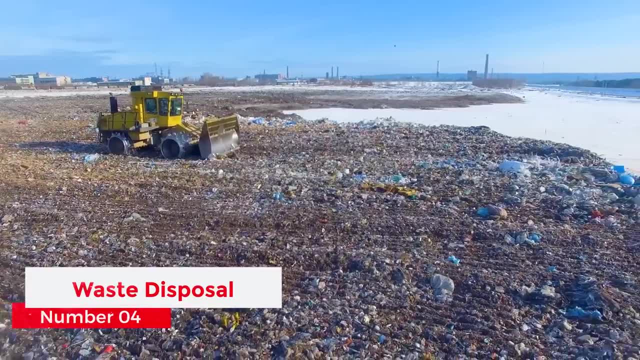 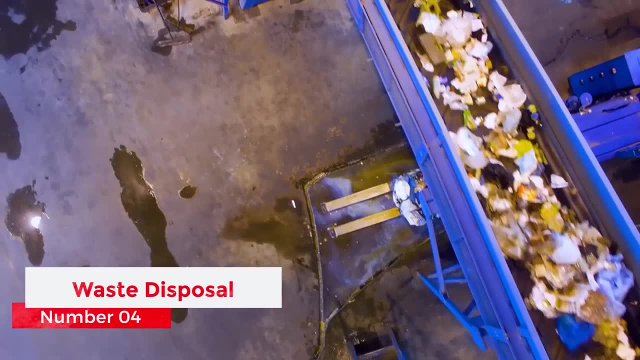 the oceans. While this helps reduce the rate of atmospheric warming and climate change, it also helps reduce the amount of CO2 released by human activities, creating a global crisis of waste disposal. Developed countries are notorious for producing excessive waste or garbage and dumping their waste in the oceans in less developed countries. Removal of garbage. 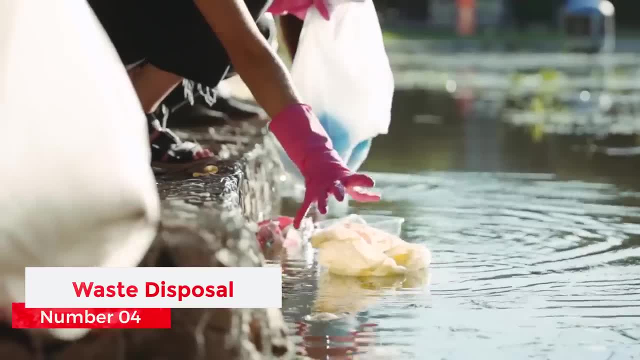 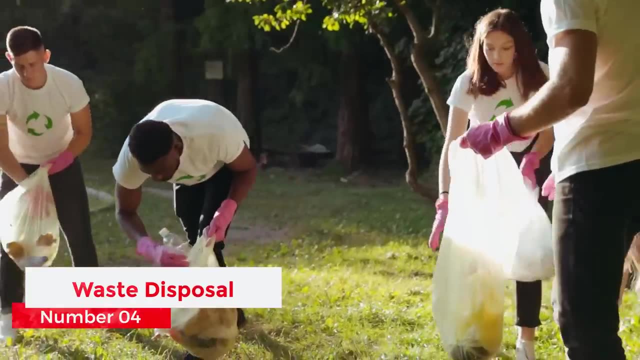 into a landfill can cause leaching of contaminants into soil and water. It also leads to the emissions of toxic gasses in the environment. Waste management has become a necessity now. Reduce, Reuse, Recycle. We should reduce our packaging purchase. minimize toxicity, then reuse bags, containers and 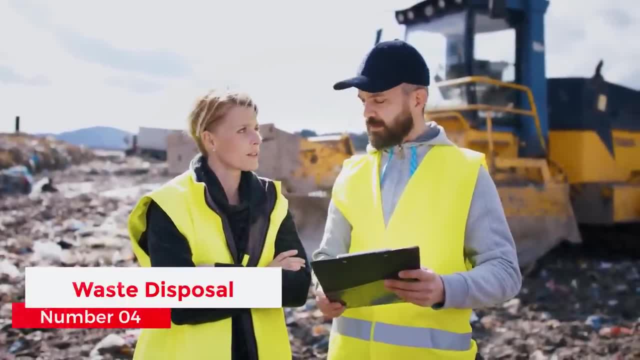 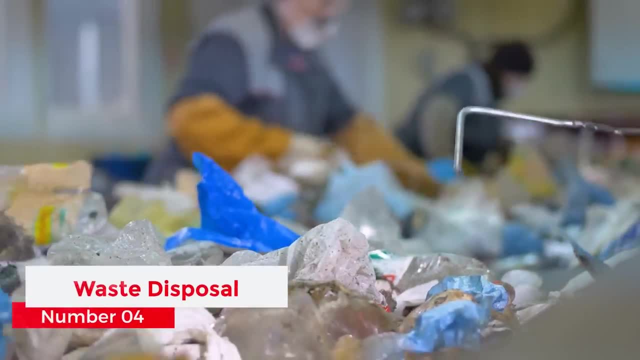 other items. • We should also start recycling. Many of us have tools and other things that we don't use regularly. Consider sharing them with your neighbors and friends. Renting is also a great option to consider. 3 – Overpopulation. • The human population continues to grow. 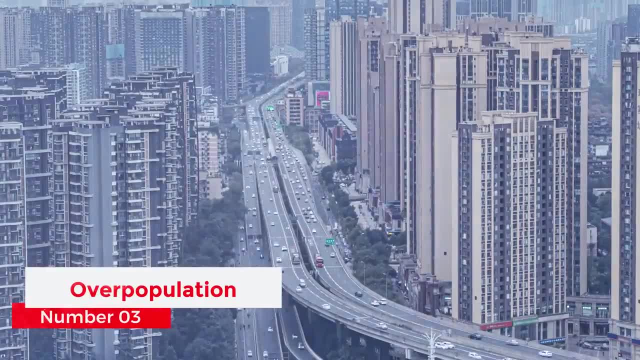 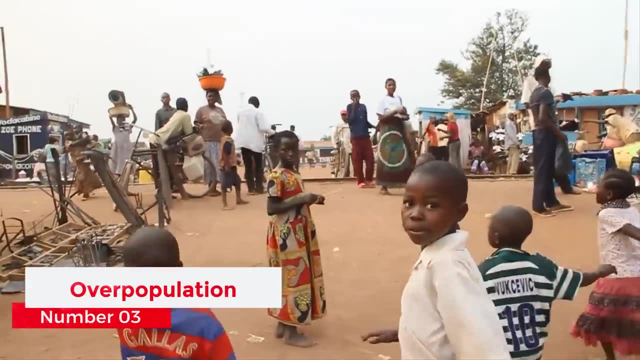 rapidly. worldwide. Humanity entered the 20th century with 1.6 billion people. Right now we're about 7.5 billion. Estimates put us at nearly 10 billion by 2050.. More people mean an increased demand for food, water, housing, energy, healthcare, transportation. 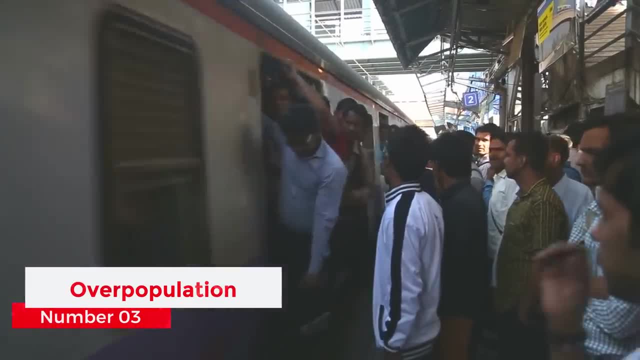 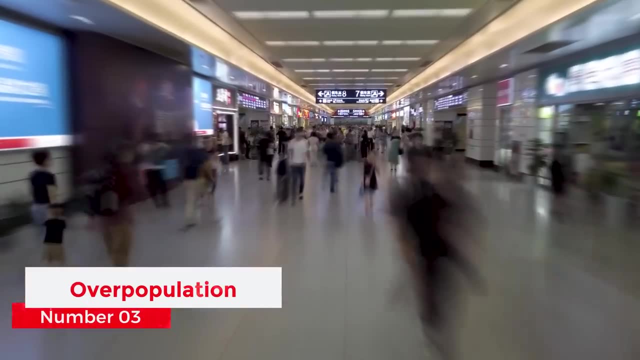 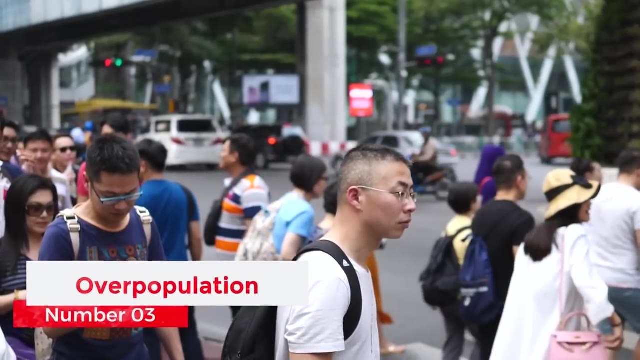 and more. All consumption contributes to ecological degradation, increased conflicts, a high unemployment rate and a higher risk of large-scale disasters like pandemics. Having a better education, like awareness of family planning and knowledge of sex education, is an effective solution to solve the overpopulation in the world. 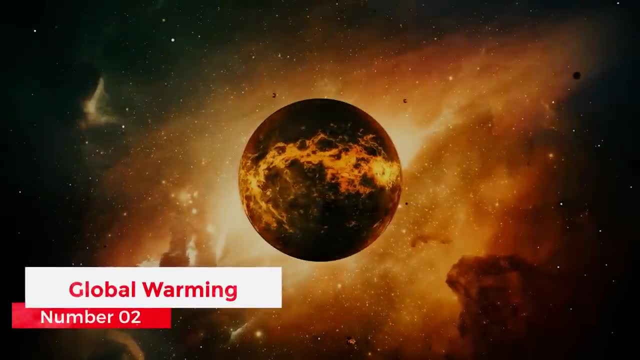 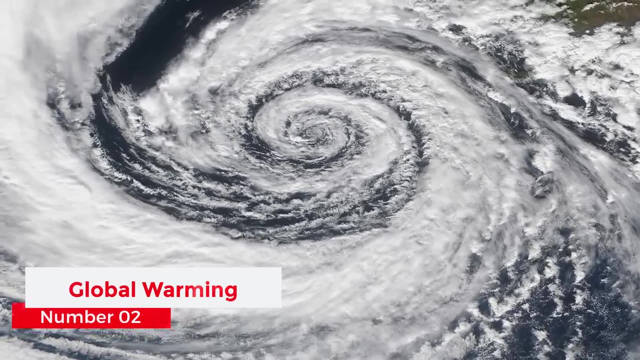 2 – Global Warming. • Global warming occurs when carbon dioxide, CO2, and other air pollutants collect in the atmosphere and absorb sunlight and solar radiation that have bounced off the Earth's surface. Climate changes like global warming are the result of human practices, like the emission 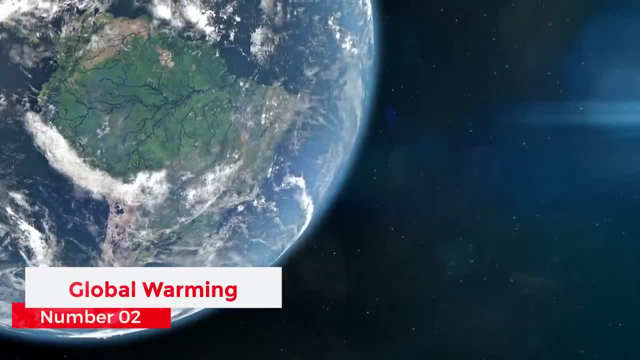 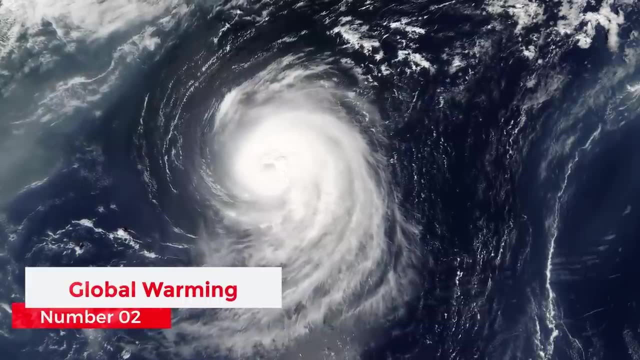 of greenhouse gases. This leads to rising temperatures of the ocean and the Earth's surface, causing natural disasters that include flooding, melting of polar ice caps, rising sea levels and unnatural precipitation patterns such as flash floods, hurricanes, wildfires, drought, excessive snow or desertification. 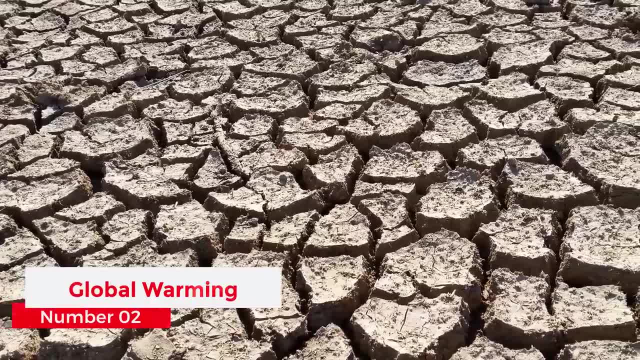 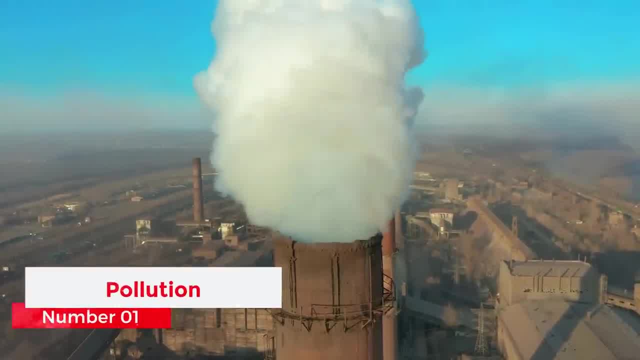 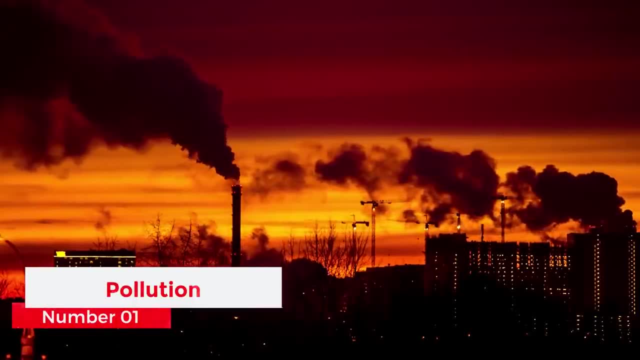 • 3. become crucial to control these carbon emissions by changing our habits. 1 – Pollution • There are seven key types of pollution – air, water, soil, noise, radioactive light and thermal. These are primary causes that affect our environment in many ways.